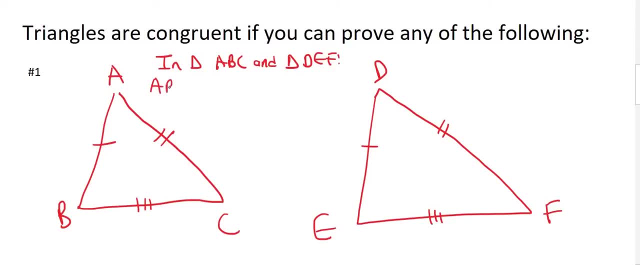 you would need to say three things. So we would say AB is the same as ED or DE, and the reason for that would be given. Then you would say, for example, that AC is equal to DF, So the reason is given. And then you would say BC is the same as EF. And you guessed. 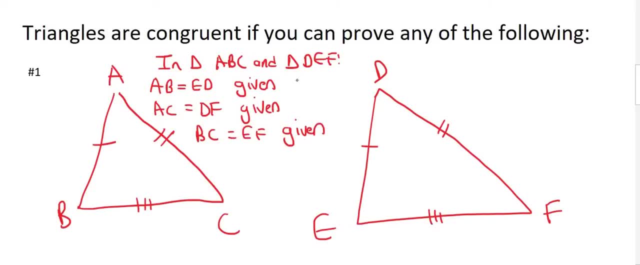 it That's going to be given. You could then say: because you have three things over there. you could then say: therefore, triangle ABC is congruent. Now, guys, congruent has three lines going this way, Okay, And then you would say DEF, And your reason for that would: 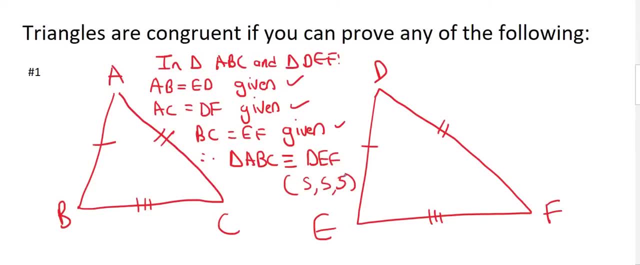 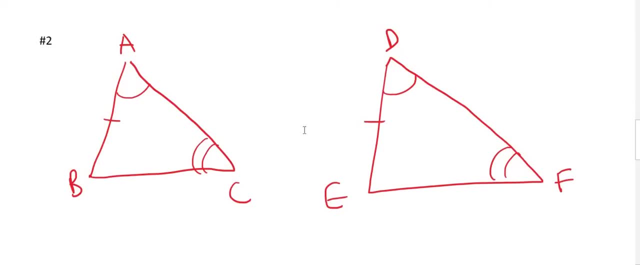 be side, Side, Side, Side, So you would say SSS, And that is how you do this in an exam. There is other ways that you could prove that two triangles are congruent, And this is the second method. So here we can see that this side is the same as this side. This angle is the same. 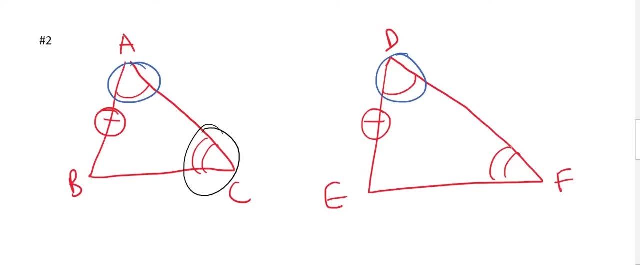 as this angle And this angle is the same as this angle. So in a test you would answer this as follows: Alright, you know, ANGLE CONFERใหL portfolio again. we just gave it two letters And if 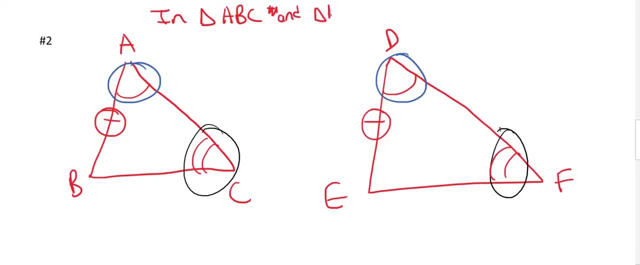 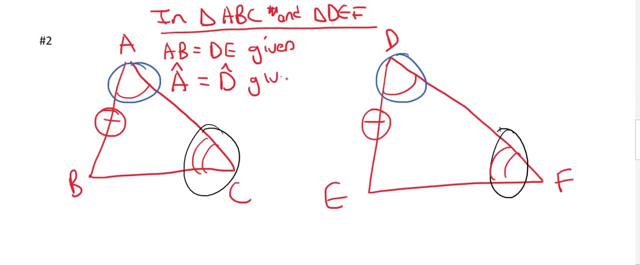 Vanderhal Z, attorney. Vanderhal Z, attorney, is equal to angle F and that's also given. and so that's three things: one, two, three. and so you could say: therefore: triangle ABC is congruent with three lines to DEF, and your reason for this one is not. 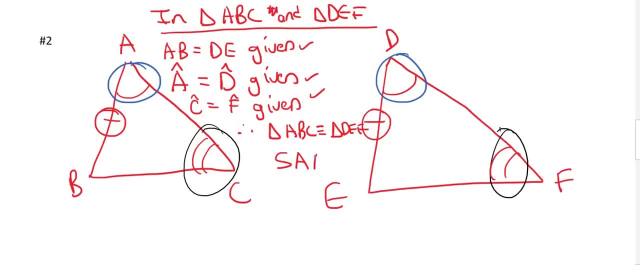 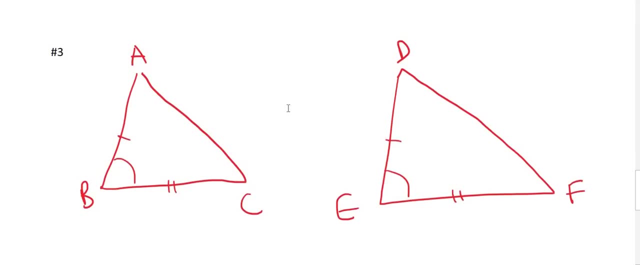 SSS, it's going to be SAA. what that means is you used a side and then you used two angles. Moving on to method number three, here we can see what's the same in these two triangles. so I'm going to quickly go and fill this in. so we'd say in triangle ABC and triangle DEF. that just lets the teacher 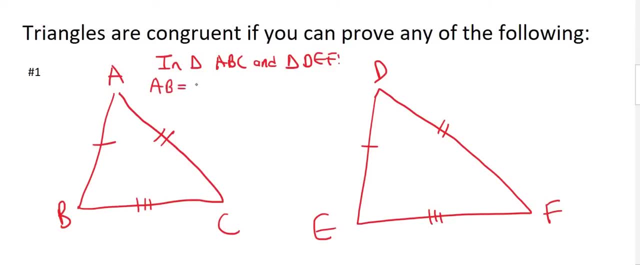 need to say three things. So we'd say AB is the same as ED or DE, And the reason for that would be given. Then you would say, for example, that AC is equal to DF, And the reason is given. And then you would say BC is the same as EF, And you guessed it, That's. 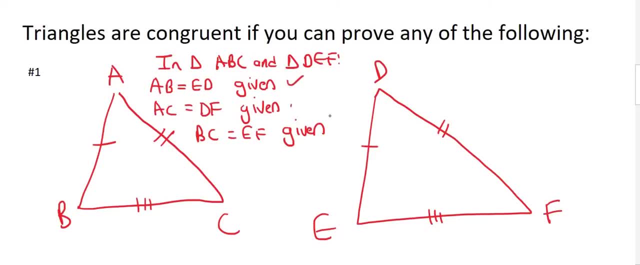 going to be given. You could then say: because you have three things over there. you could then say: therefore, triangle ABC is congruent. Now, guys, congruent has three lines going this way. Okay, And then you would say DEF, And your reason for that would be side A. 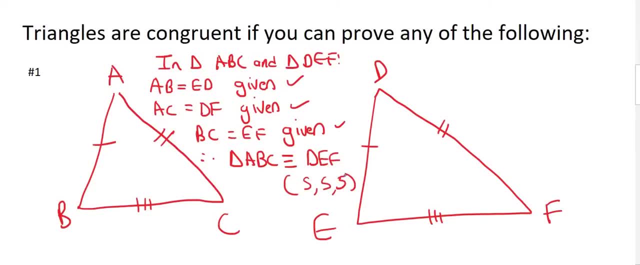 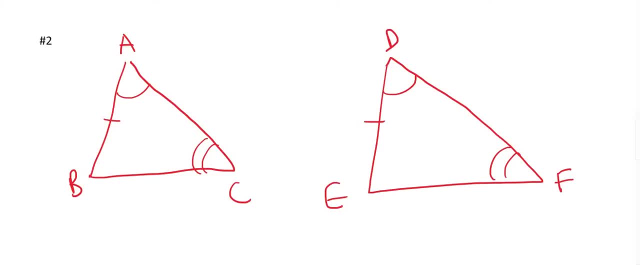 side, side, side. So you would say SSS, And that is how you do this in an exam. There is other ways that you could prove that two triangles are congruent, And this is the second method. So here we can see that this side is the same as this side. This angle is the 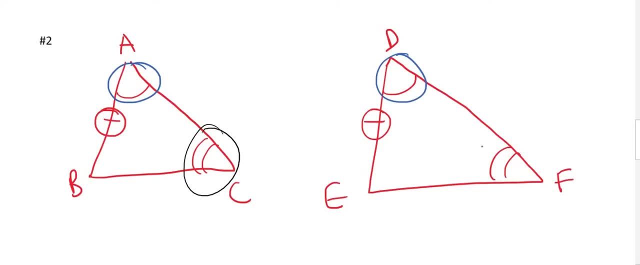 same as this angle And this angle is the same as this angle. So in a test you would answer this as follows: You would first say which triangle is congruent, And then you would say IN triangle A, B, C and triangle DEF. You could then put a line like that: 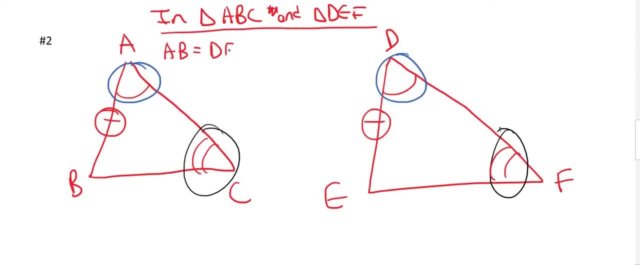 And then you could say: AB is equal to DE. Why is that? They gave that to you. So you can say given. Then we can say angle. So you would say angle A with a little arrow on the side. That means angle is the same as angle D And that's given. And then you could say: 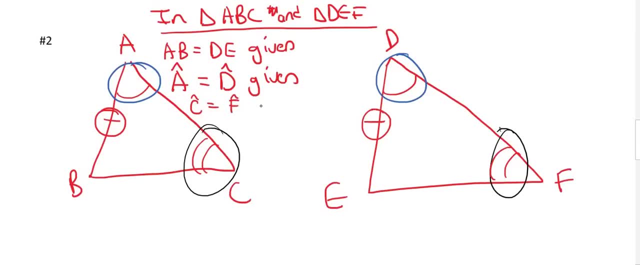 angle C is equal to angle C, And that's given. And then you could say: angle C equal to angle to angle F, and that's also given. And so that's three things: 1,, 2, 3.. And so you could say: 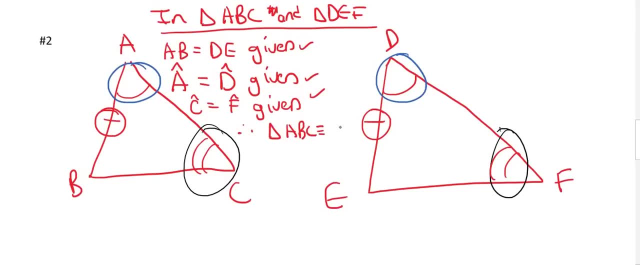 therefore, triangle ABC is congruent with three lines to DEF, And your reason for this one is not SSS, it's going to be SAA. What that means is you used a side and then you used two angles. Moving on to method number three, Here we can see what's the same in these two triangles. So 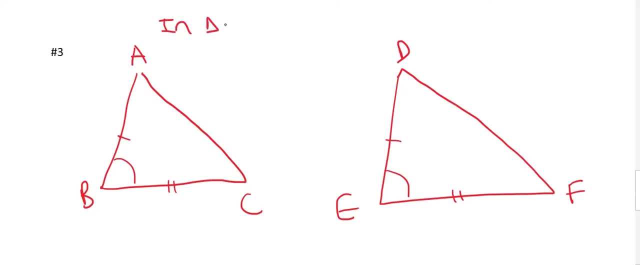 I'm going to quickly go and fill this in. So we'd say in triangle ABC and triangle DEF. that just lets the teacher know which triangles you're working in. Then you could say: AB is equal to DE, Y, it's given. BC is equal to EF, and that's given. And then the angle B is the same. 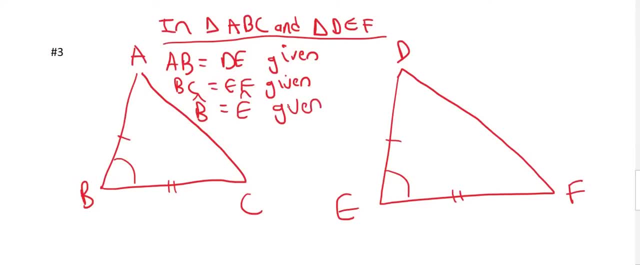 as the angle E, and that is also given. So therefore, we've got one, two, three things we can say. triangle ABC is congruent to triangle DEF. Now, your reason for this one is very important. This is where teachers like to try and trick you out. We have two sides and the angle is in between. 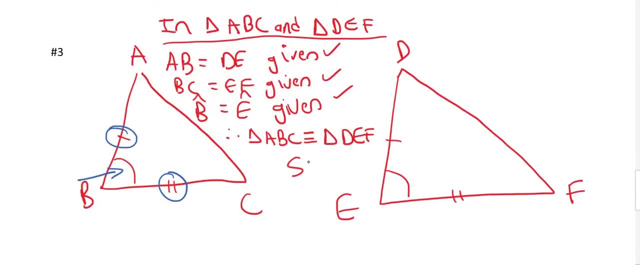 them. So for this one you could say: side, angle, side in a bracket. Guys, if the angle is not in between the two sides, then you've got to say triangle ABC is congruent to triangle DEF. So if the angle is not in between the two sides then it's not congruent. Okay, so you never want to. 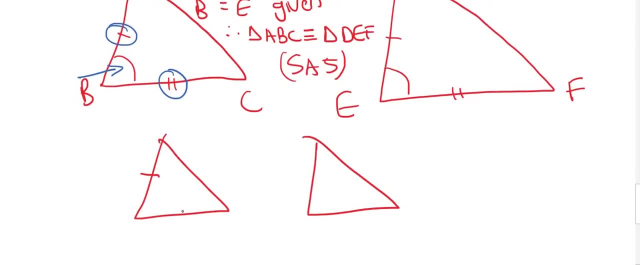 end up with something like this, For example, you never want to have a side. Well, let me first just draw this out: You never want to end up with a situation like this, Because- have a look here- This angle is not in between the two sides. If it was, it would be over here. So these two triangles. 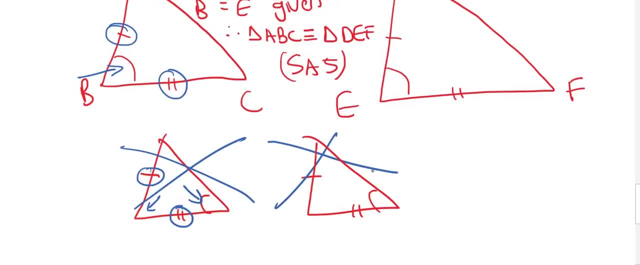 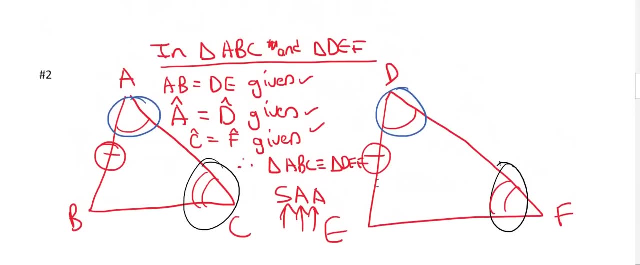 are not congruent. So the angle must be in between the two sides. So if it was, it would be over here. So the angle must be in between the two sides. But, Kevin, you didn't mention that earlier when we were doing number two. Yes, guys, when you have a side and two angles, then it doesn't matter. 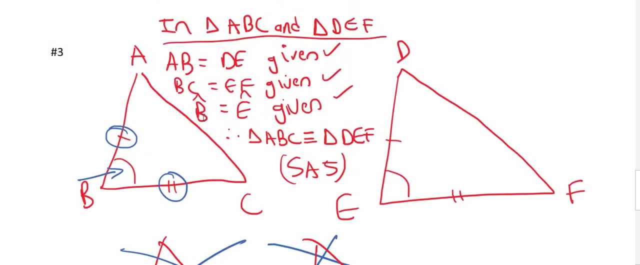 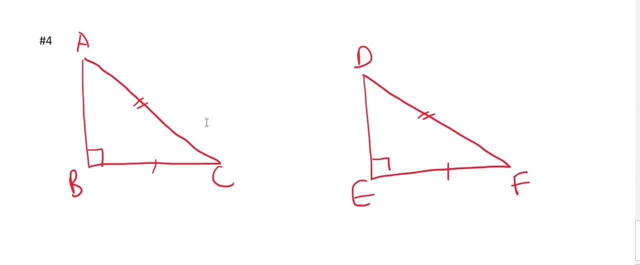 But when you have two sides and an angle, then you have to be careful. Then your angle has to be in between the two sides, And the last method that you can use for congruency is the following: So this is where you could also get confused. You would first say in triangle ABC. 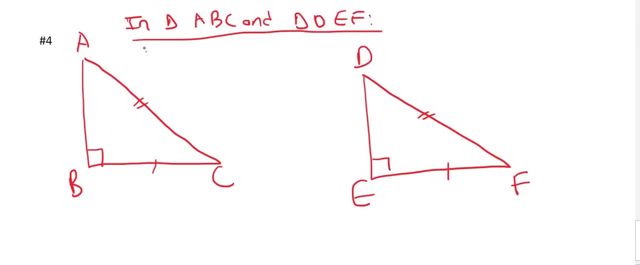 and triangle def. you could maybe say that bc is the same as ef. why? because that's given. you could then say that ac is equal to df, and that's also given. then you could say that this angle, which is angle b, is the same as angle e, and that's also given. then you might say, therefore, triangle abc. 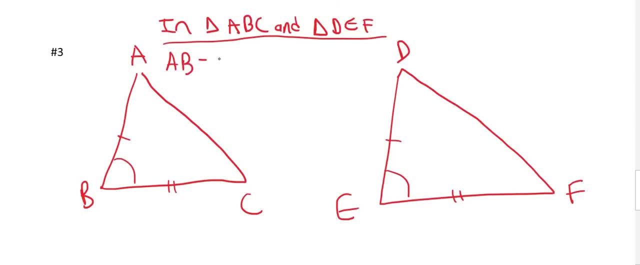 know which triangles you're working in. then you could say: AB is equal to DEY, it's given. BC is equal to EF, and that's given. and then the angle B is the same as the angle E, and that is what we're going to do. So we're going to say triangle AB is equal to DEY, and that's given. 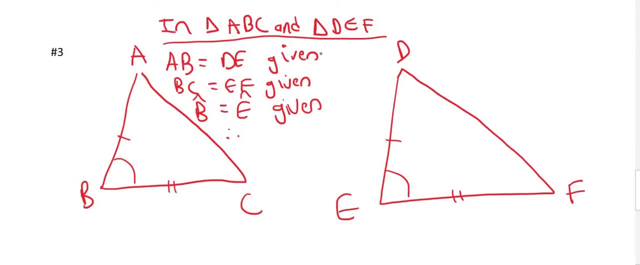 and that's given. and then the angle B is the same as the angle E, and that is what we're going to do, also given. so therefore, we've got one, two, three things we can say. triangle ABC is congruent to triangle DEF. Now, your reason for this one is very important. this is where teachers like to. 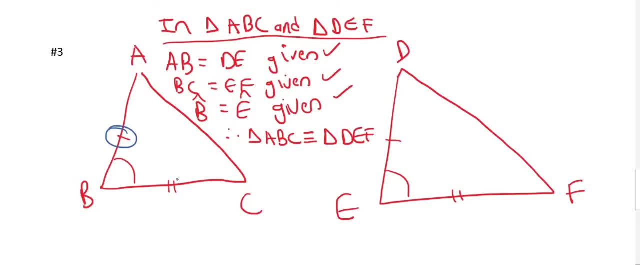 try and trick you out. We have two sides and the angle is in between them. so for this one you could say side angle, side in a bracket. Guys, if the angle is not in between the two sides, then it's not congruent. okay, so you never want to. 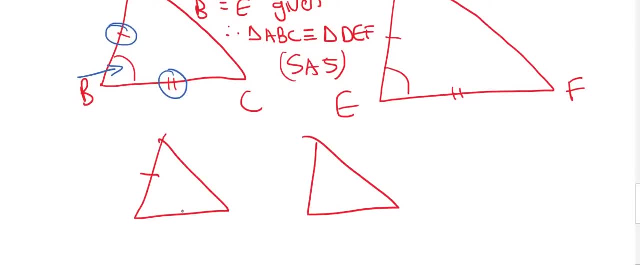 end up with something like this, for example, you never want to have a side. well, let me first just draw this out: you never want to end up with a situation like this because- have a look here- this angle is not in between the two sides. if it was, it would be over here. so these two triangles. 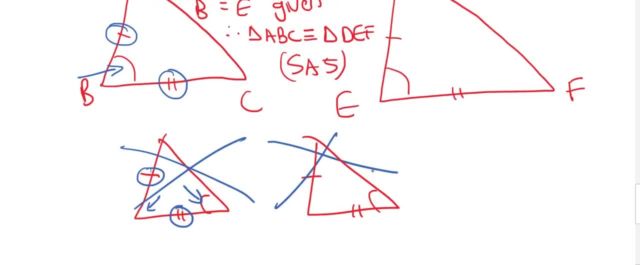 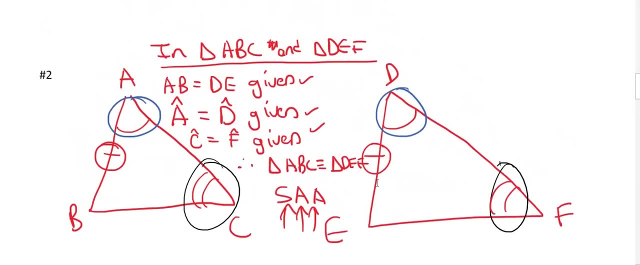 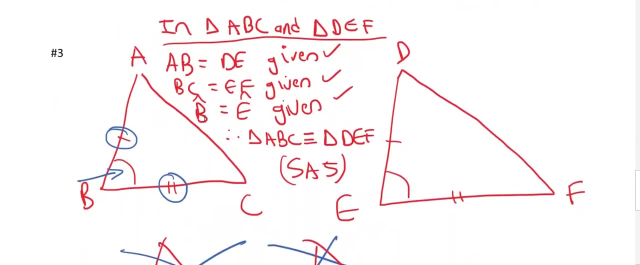 are not congruent. so the angle must be in between the two sides. but, Kevin, you didn't mention that earlier when we were doing number two. yes, guys, when you have a side and two angles then it doesn't matter, but when you have two sides and an angle then you have to be careful. then your angle has. 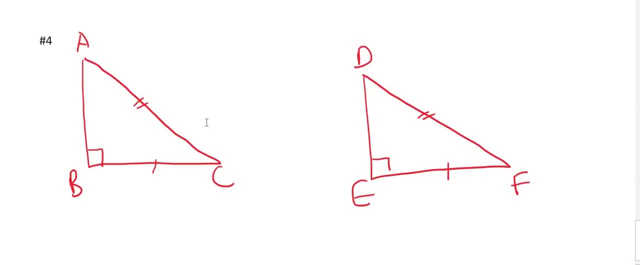 to be in between the two sides, and the last method that you can use for congruency is the following: so the angle must be in between the two sides and the angle must be in between the two sides and the. this is where you could also get confused. you would first say in triangle ABC and triangle DEF. 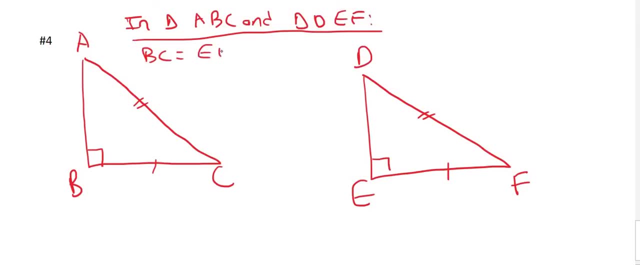 you could maybe say that BC is the same as EF. why? because that's given. you could then say that AC is equal to DF, and that's also given. then you could say that this angle, which is angle B, is the same as angle E, and that's also given. then you might say therefore: